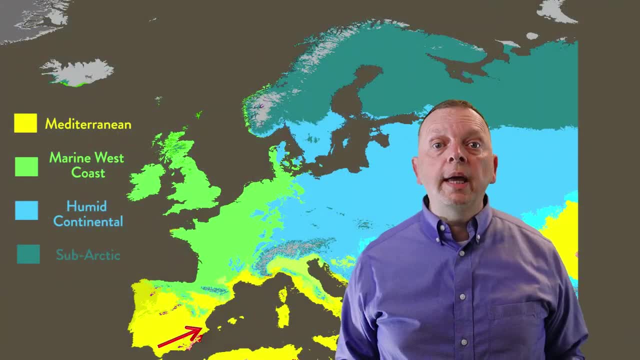 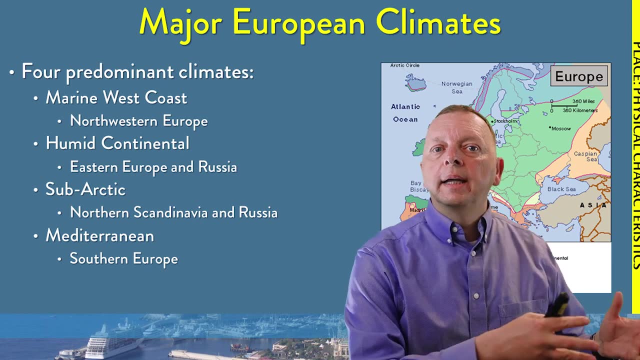 Now, if we go down in the southern portion of Europe around the Mediterranean Sea, we get a climate that is actually named after it, the Mediterranean climate. This is the same climate we find in Southern California. In fact, in the 1960s, a lot of Clint Eastwood western movies. 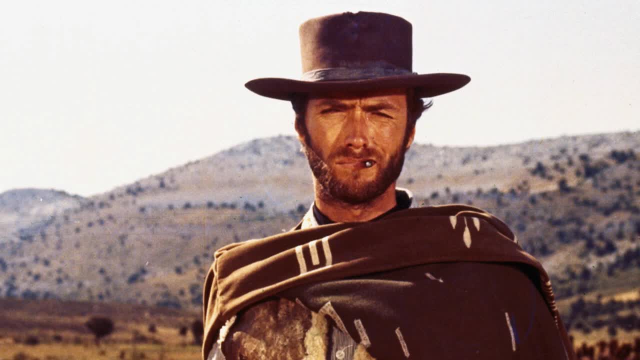 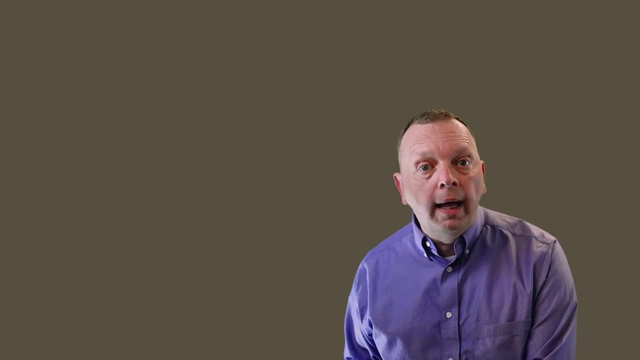 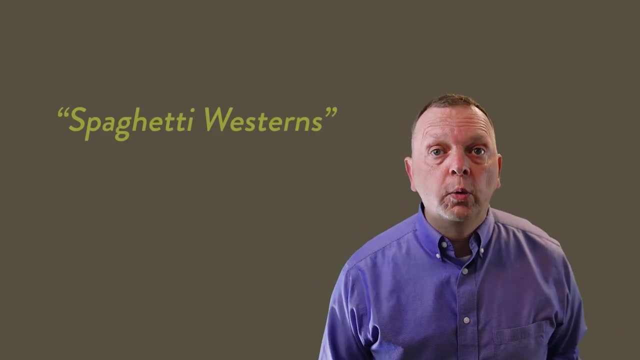 were actually shot in Southern California, were actually shot in Southern California. They were actually shot in Italy, because Italy has this Mediterranean climate which is the same as the American Southwest. These westerns actually were called spaghetti westerns, So by now we should be able to describe the significant landforms of Europe. 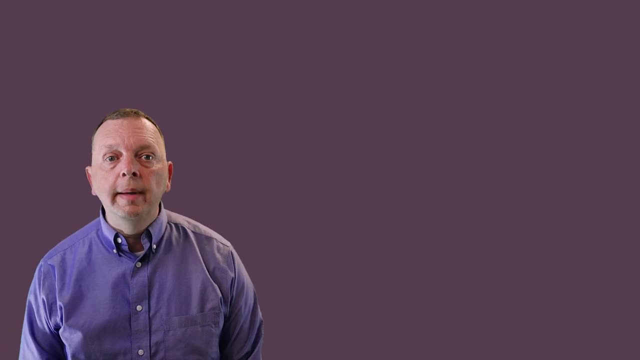 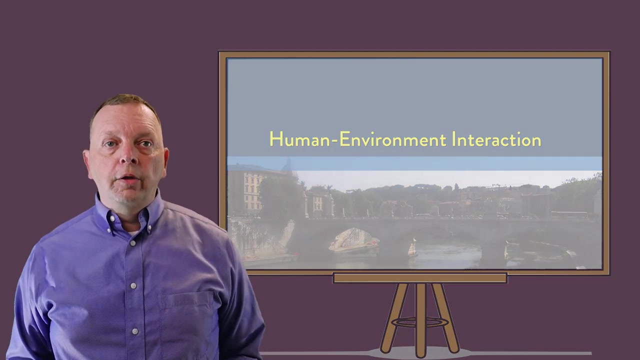 We talked about those in our last lesson and we just talked about its climate. So now let's look at some of the ways that mankind has interacted with its environments in Europe, And one example is what we find in the Netherlands, A problem that the Dutch have- and the Dutch is the term we use for someone from the Netherlands- 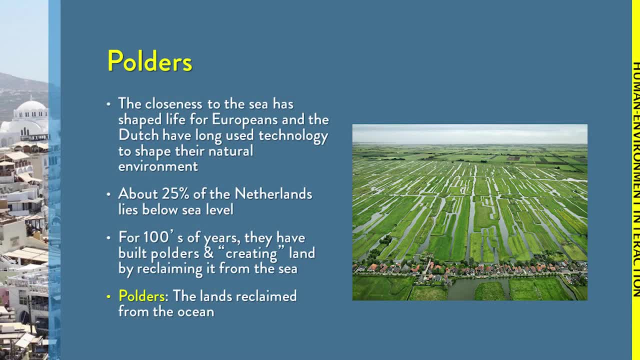 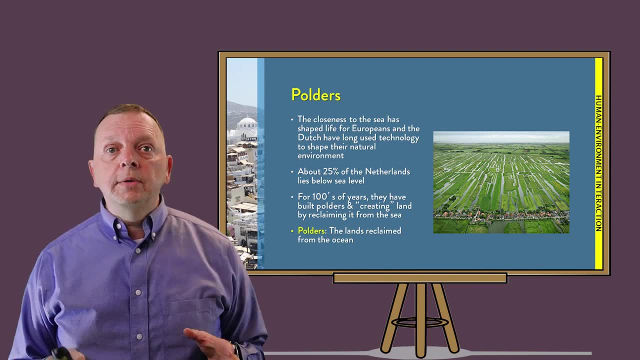 is that 25% of the Netherlands actually lies below sea level. This is quite problematic for a country that lies right on the coast of the North Sea. Now we often think of dikes or dams in the Netherlands to prevent being flooded, but it's far more than that. For hundreds of years, the Dutch have actually 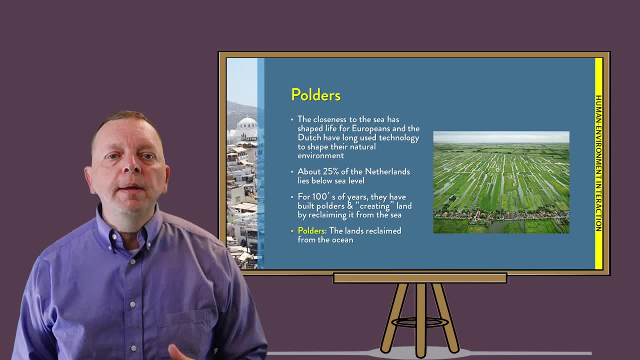 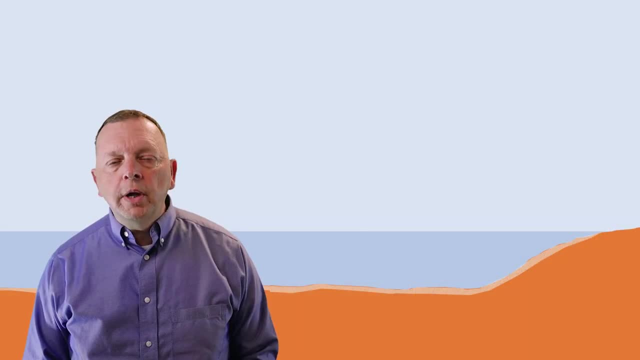 been reclaiming land from the sea. Literally, they've been making more land out of what used to be the sea. They do this through what they call the polders. The first step of the polders is building a dam. Then what they do is they pump out water out of the area that's being reclaimed. 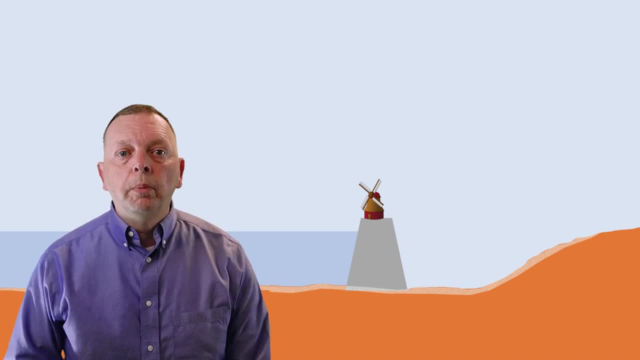 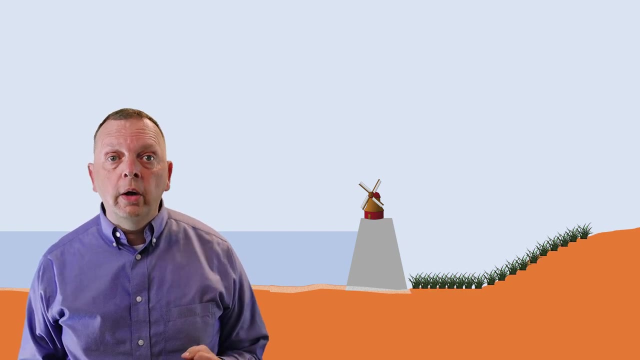 Then, when the water is removed from that area, then what they'll do is they'll plant plants that actually absorbs the salt out of the ground. After five years of letting the plants leach the salt out of the soil, this land is actually ready to be used by the Dutch Today. one-sixth, 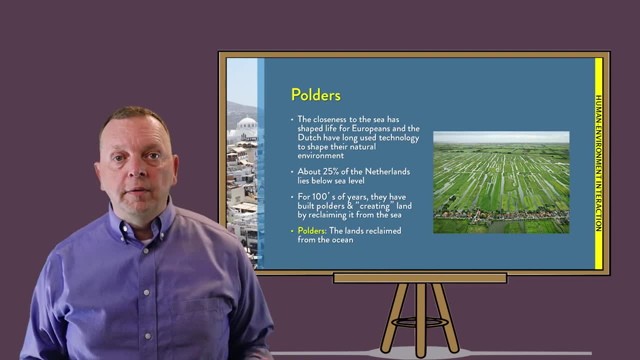 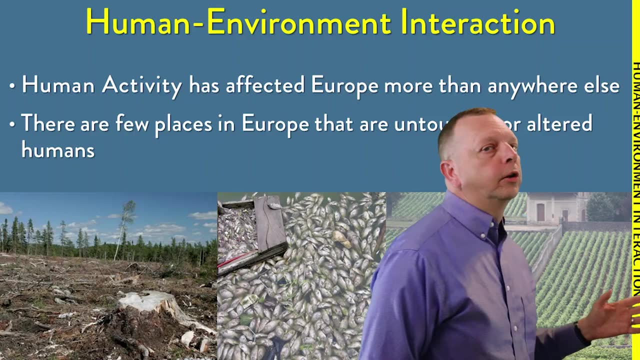 of the land of the Netherlands is land that has been reclaimed from the sea. These two maps here shows us how much land has actually been claimed by the Dutch. Now, when we look at how long mankind has been in Europe, it's easy to understand how Europe has. 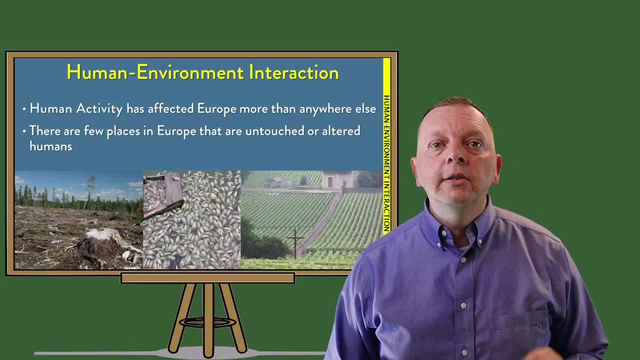 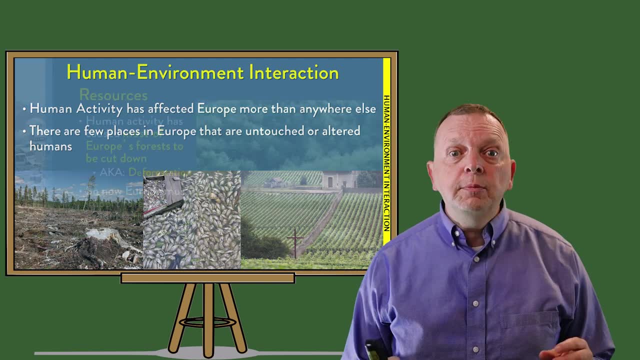 been affected for mankind over a long, long time. Today, there are few places in Europe that have been untouched or changed by humans. One of the effects of mankind's activities has been deforestation, which is the cutting down of Europe's trees. Trees have been cleared to make 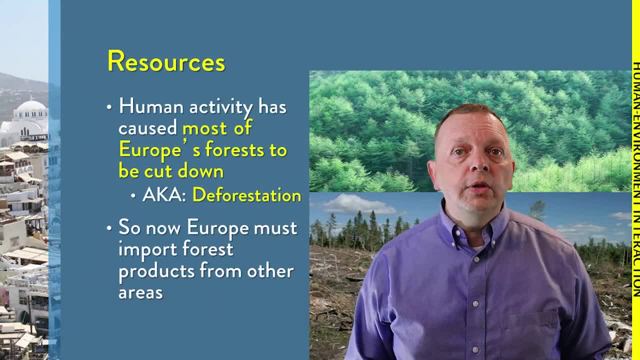 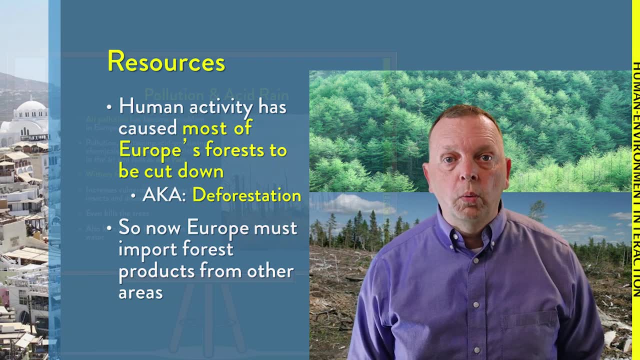 room for cities, roads and to get out resources. Of course, they've also been cut down for lumber. So after as many years, today Europe and the rest of the world have been able to import forest products from other regions of the world. 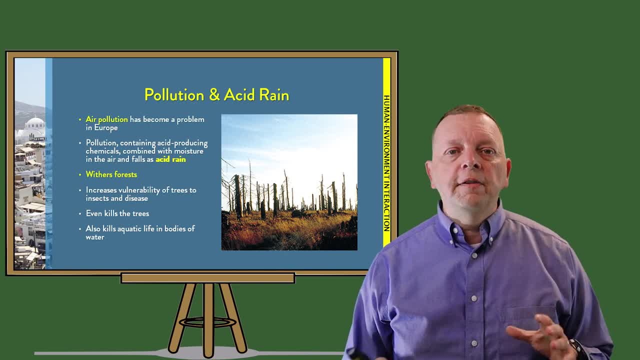 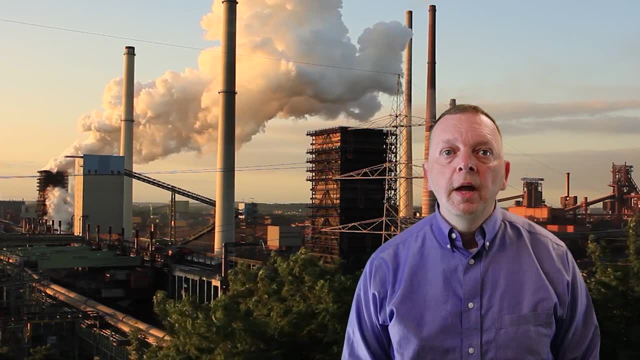 Pollution has also been a major reason for the loss of so much of Europe's forests. Because of factories and cars, air pollution in Europe has become an issue for not only its people but for its forests. The resulting air pollution in the air combines with moisture and then falls down as 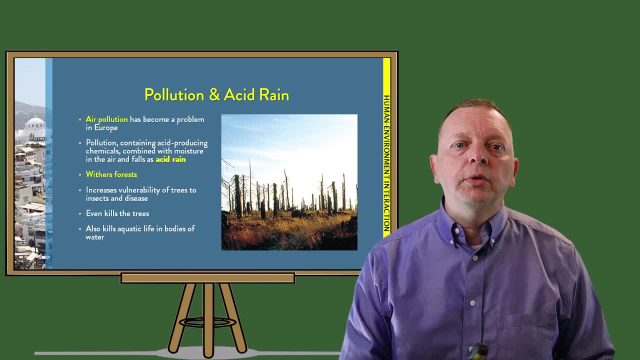 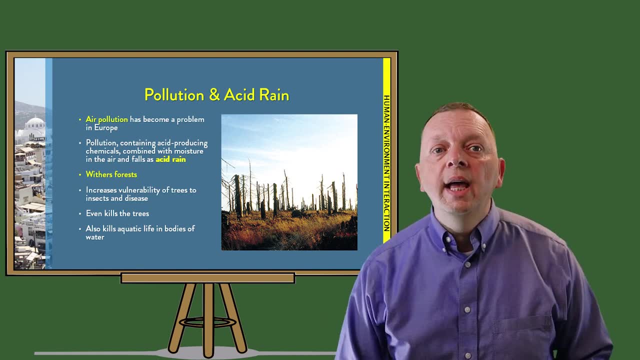 acid rain. This acid rain then weathers the forests, making the trees more vulnerable to insects and disease. After a while, the trees die off. Acid rain also runs off into the rivers and streams and can kill the aquatic life there. The effects are especially harsh in Eastern Europe, where coal 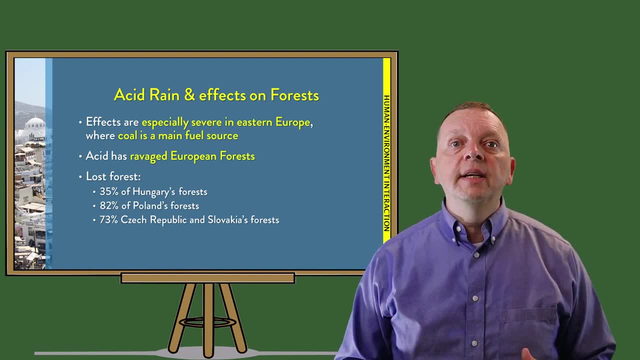 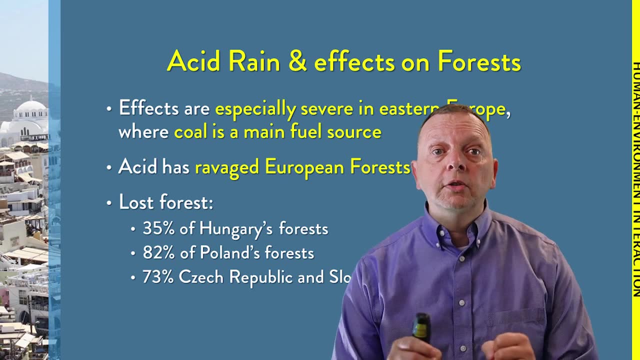 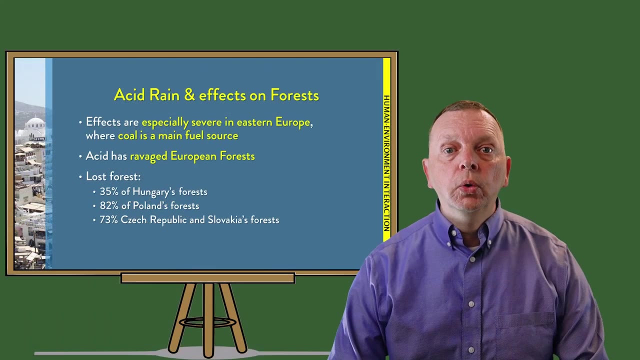 is used more than any other forms of energy. Thus, it is the forests in Eastern Europe that have been most affected: 35% of Hungary's forests, 73% of the Czech Republic and Slovakian forests and an astonishing 82% of the Polish forests have been lost due to this acid rain problem. Now, while 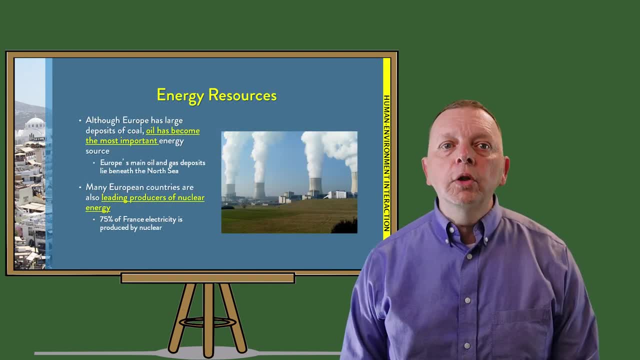 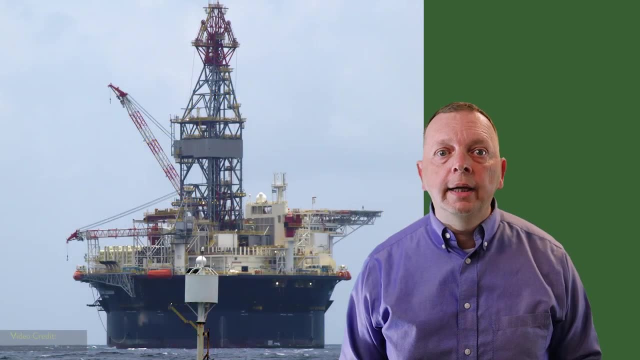 coal is the primary source of electric energy in Eastern Europe. for the rest of the world, oil and natural gas is the important energy source. Fortunately for some countries such as Norway and the United Kingdom, they have sizable oil and natural gas deposits that lie underneath. 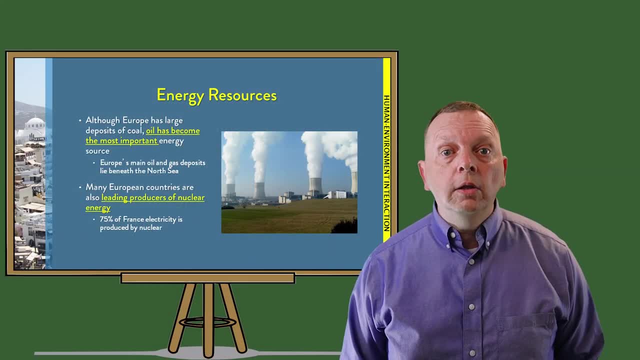 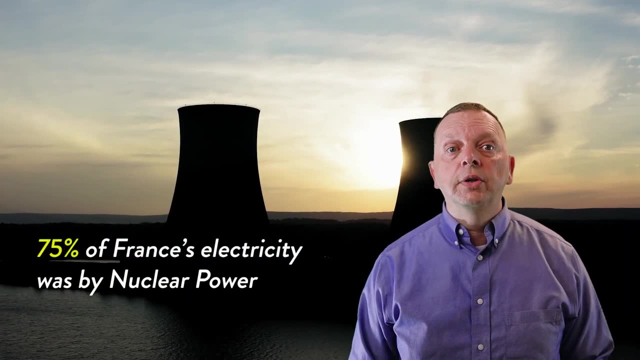 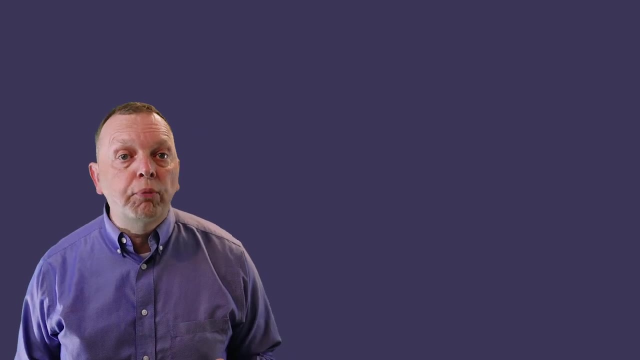 the North Sea. Russia also has a very large oil reserves, And other European countries are leading producers of nuclear energy. 75% of France's electricity is produced by nuclear power plants like these shown here. But nuclear energy can have drawbacks if not properly watched after. 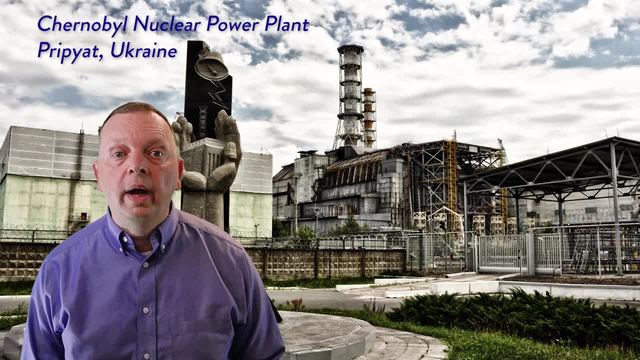 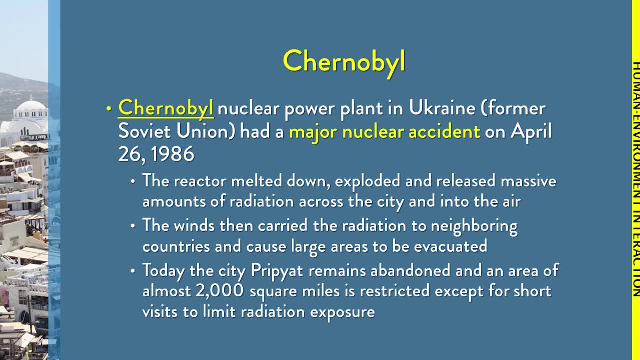 In 1986, the Soviet Union found this out the hard way in a place known as Chernobyl. Now, due to a number of human errors, the reactor melted down, exploded and released massive amounts of radiation across the city and into the air. The winds then carried the radiation to neighboring